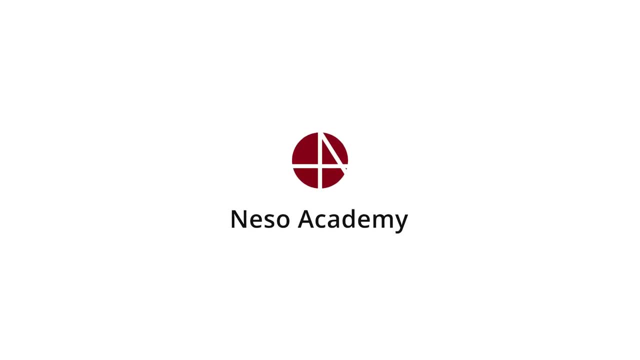 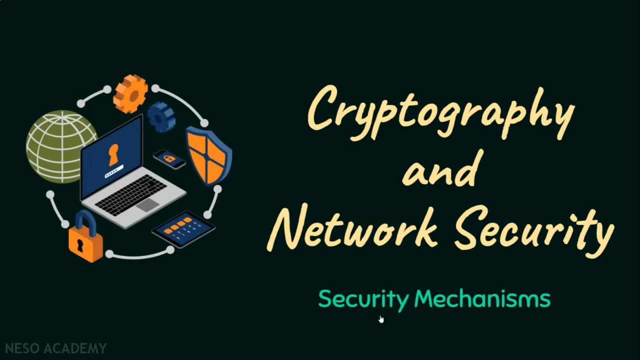 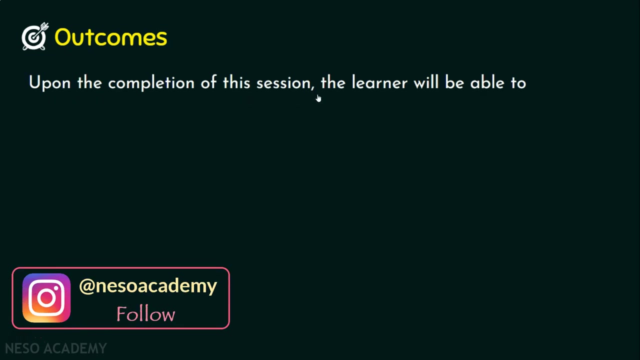 In the last presentation we have seen about security services. In this presentation, we are going to focus on security mechanisms. As usual, let's start the session with the outcomes. Upon the completion of the session, the learner will be able to understand various 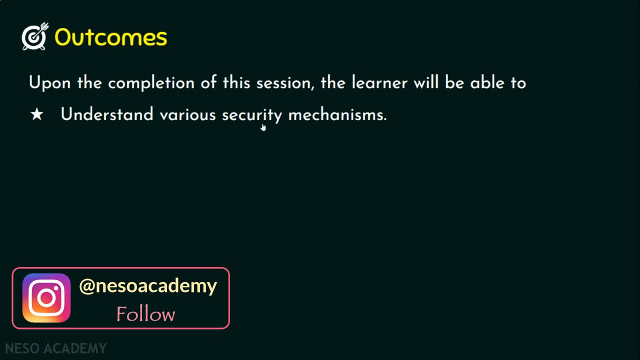 security mechanisms. In today's lecture we are going to mainly focus on various security mechanisms. Before stepping into what security mechanisms, let's see the OSA security architecture We know the OSA security architecture deals with the three key components. Number one: 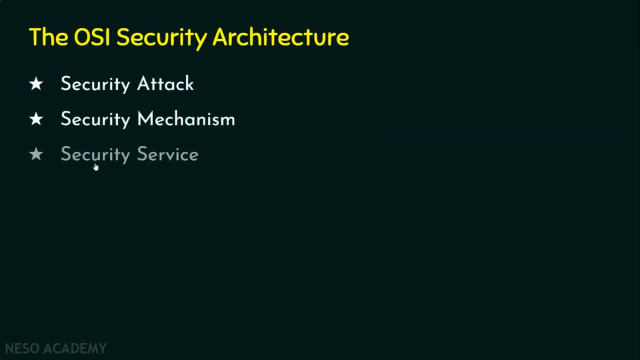 security attack, Number two security mechanism And number three, security services. In the previous presentations we have seen about security attacks and security services. Now we are going to focus on security mechanism. What is the security mechanism? We need security. 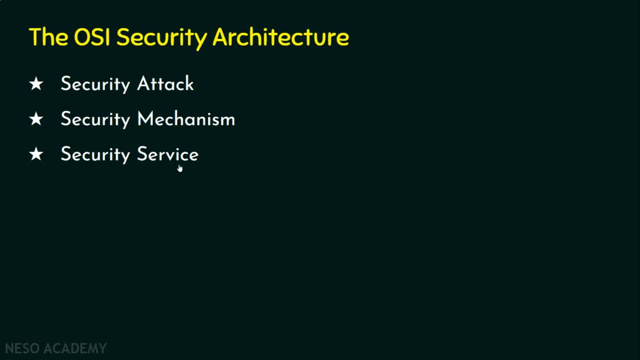 services, and these security services implement security mechanisms. So let's start the session with the security policies that are implemented by the security mechanisms. So let's dive into the topic of the day: the security mechanism. Basically, we have two types of security mechanism. 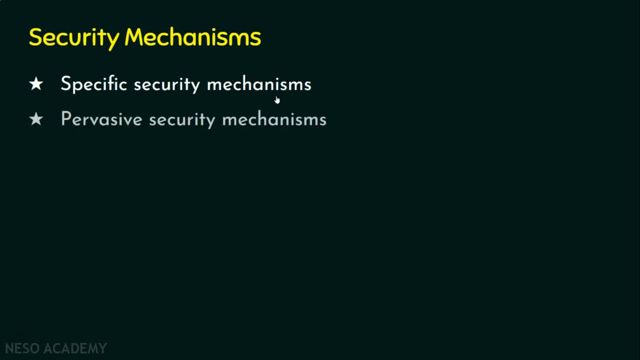 Number one: specific security mechanisms And number two: pervasive security mechanisms. Let's start with the first security mechanism, the specific security mechanism. The name itself says that it is specific, So these specific security mechanisms are incorporated into appropriate protocol layers to prevent the automation of the security mechanism. So let's start with the 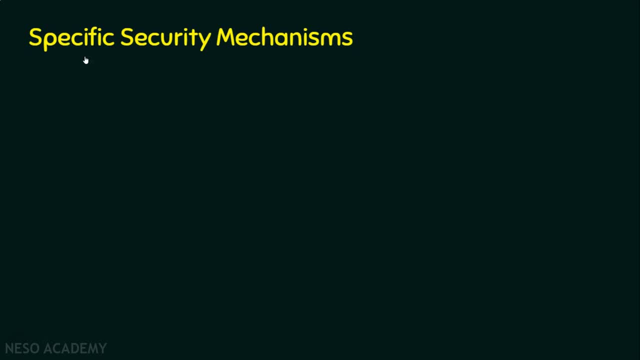 provide some of the OSI security services. We have seen various security services in the last lecture and these specific security mechanisms incorporate into protocol layers in order to provide some of the security services that we have seen. Let's see the various security mechanisms. The first one we would like to address is the encipherment. 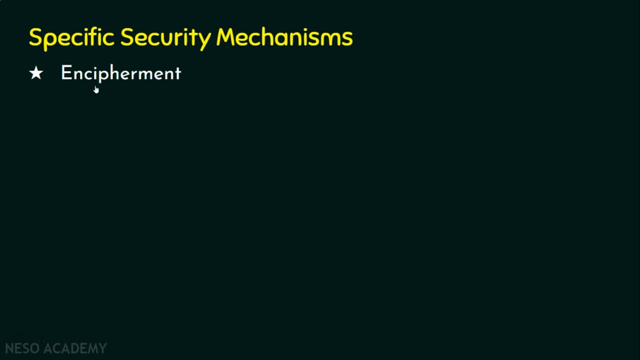 What is this encipherment? This encipherment means it is ciphering technique. If we have a plain text, we want to convert that plain text into ciphertext before sending the data to the internet, because internet has bad guys- the attackers- So we want to ensure that we are getting confidentiality. 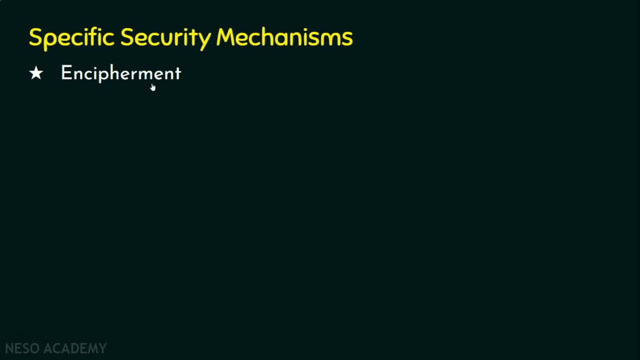 We want to achieve that. we get the service confidentiality, or data confidentiality. How data confidentiality can be achieved? It is achieved because of this encipherment, Now how this ciphertext are generated. We have a lot of mathematical algorithms that create ciphertext. As already mentioned, cryptography deals with a lot of 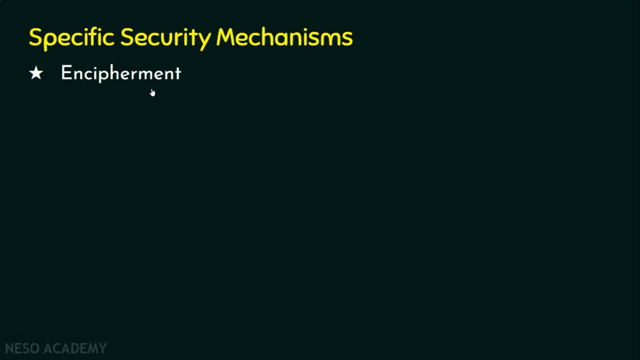 mathematical algorithms. So if we have a strong mathematical algorithm, it means the ciphertext cannot be broken as easily. one thing, So this mathematical algorithm is going to use a key. This key is the critical information in order to convert the plain text into ciphertext. 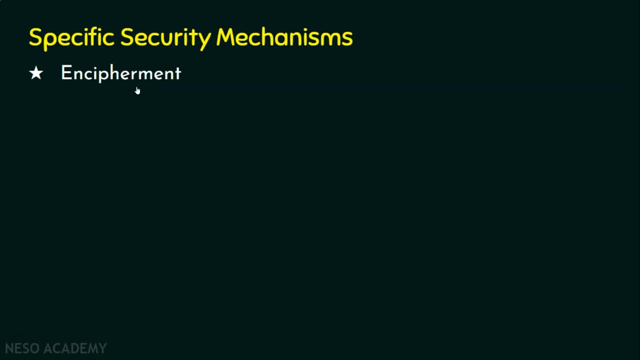 So this is about encipherment. Let's see the second security mechanism, the digital signature. The name itself says that it is going to be having a signature in order to prove the identity of the sender. Many people will confuse that the soft copy signature is called. 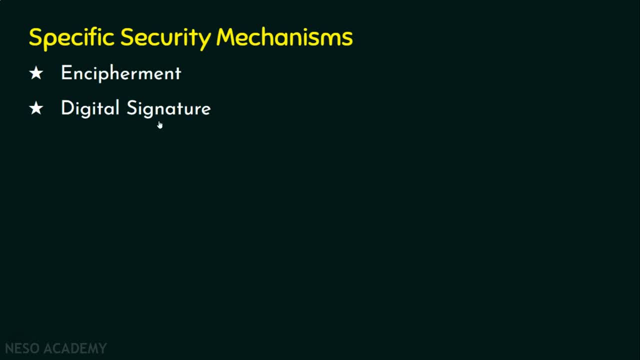 as a digital signature. As far as security systems are concerned, there will be a piece of code that is inserted to the message and this piece of code only is going to act as a signature of the sender When receiver receives it, and the receiver can understand that. 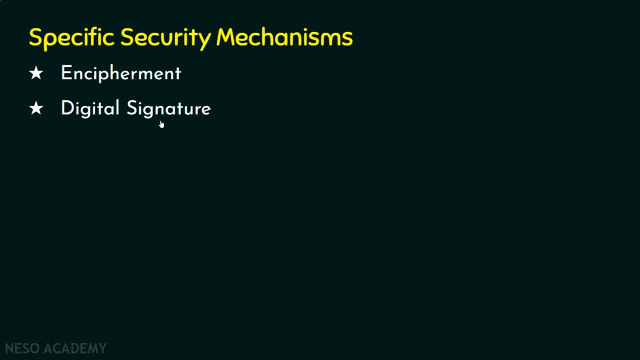 it is from the right sender. So why we need digital signature In order to prove the identity of the source? What is that actually? What security service is that Proving the right source is actually authentication. In order to have authentication, we need digital signatures. 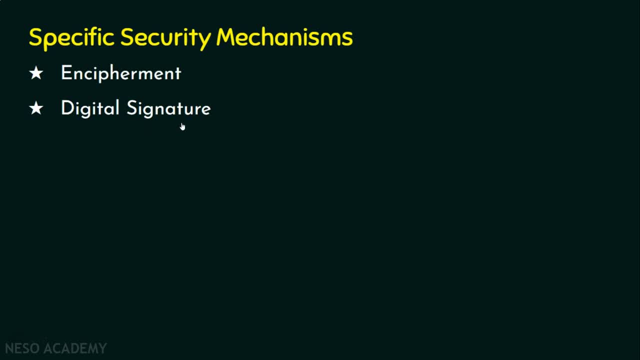 So we have seen authentication service in the last lecture. In order to get authentication service, we are using digital signatures, and this digital signatures are not only for authentication. It also provides one more service: data integrity. So it gives the assurance that the data is not modified during. 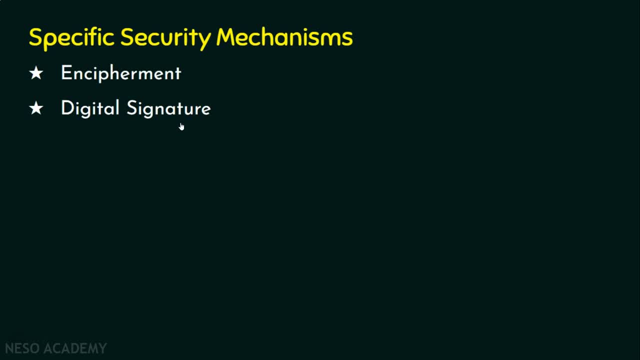 transaction. So whatever the sender is sending, that, only the receiver is receiving. that assurance is also given by digital signatures. In a nutshell, digital signature provides both authentication and integrity. Coming to the third one, the access control. This access control is also a security service. 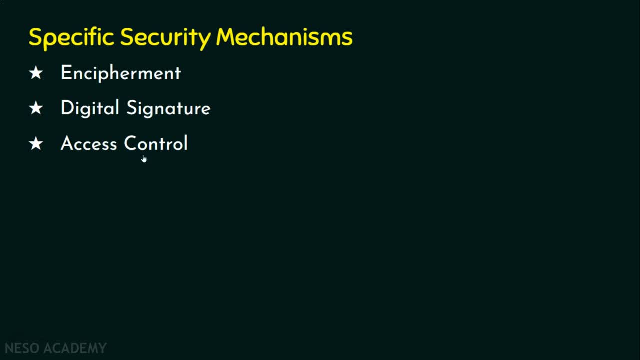 Already. we have seen this. This is giving access rights to the resources. Not all the users will be given with the same access levels or same access rights, So every user will be having their own set of access privileges. So we are going to provide access rights to the users who can access what. 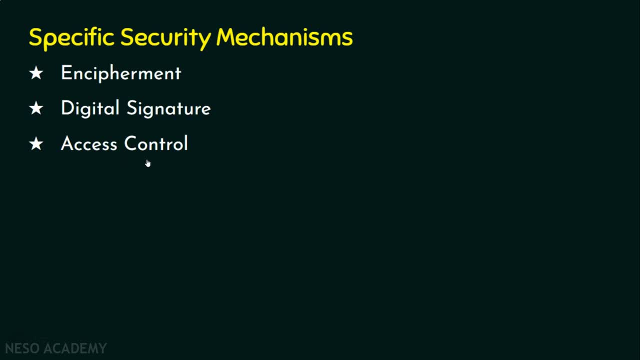 We are done with the third security mechanism. Let's now move on to the fourth security mechanism, the data integrity. We have already seen this data integrity. Whatever the sender is sending, that only receiver should receive. So we need to ensure that the data was not subjected to any 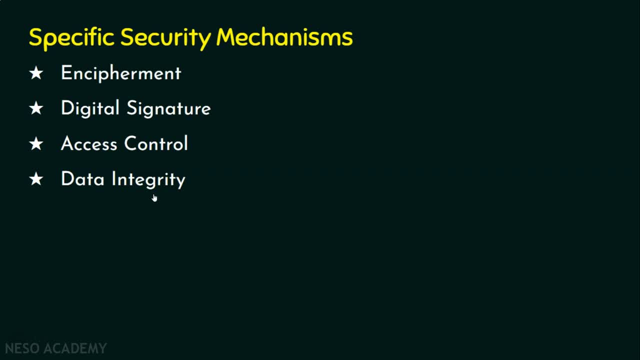 modification during transmission. If an attacker modifies the data that is being transmitted between the sender and the receiver, or between the source and the destination system, should be able to find out that. So this is actually data integrity. Coming to the next security mechanism, which is the authentication exchange. 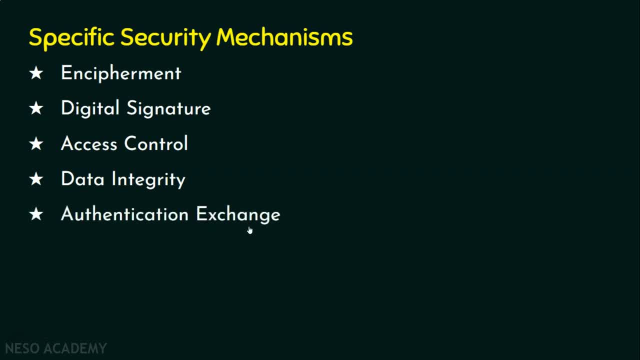 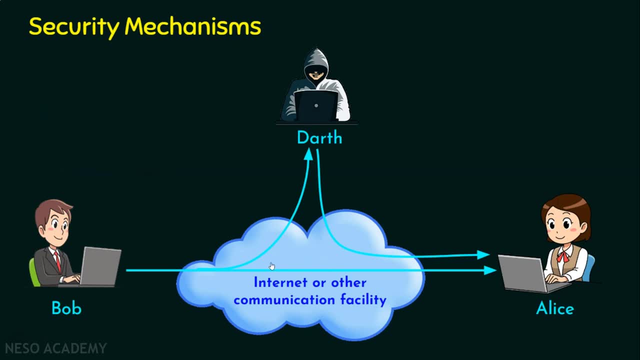 So this mechanism ensures that the identity of an entity by means of an information exchange. Let's take an example. In this example, let's assume there are two neighboring routers. Now when one router is forwarding data to the other router, the router. 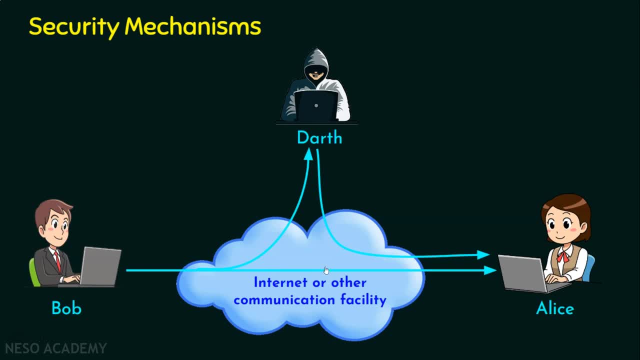 which receives the data packet or the message should confirm that the message is from the neighbor only and not from other routers. How these two routers can confirm that they are neighbors only and they are authentic nodes? It is by exchanging a small piece of information periodically so that 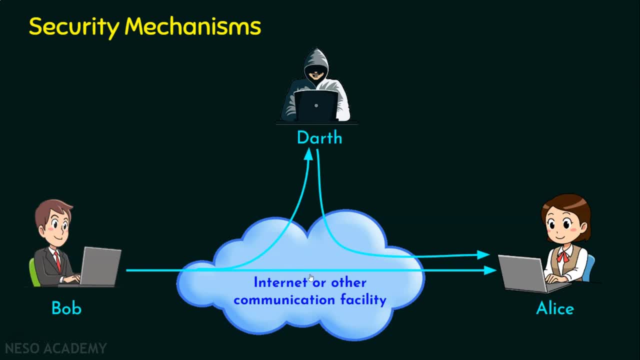 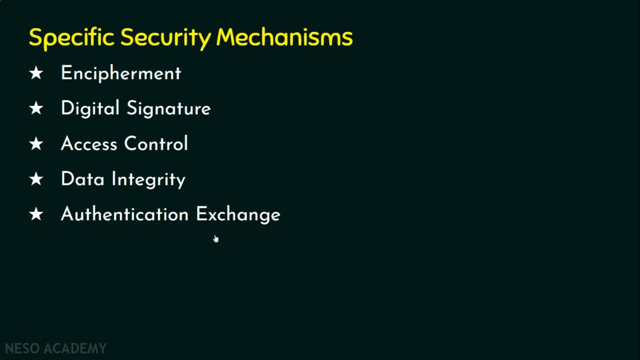 they can understand that they are the authentic nodes in the network or they are the valid or the legitimate routers in the network. So this is about authentication exchange In a nutshell. a small piece of information is going to be exchanged between entities, just for. 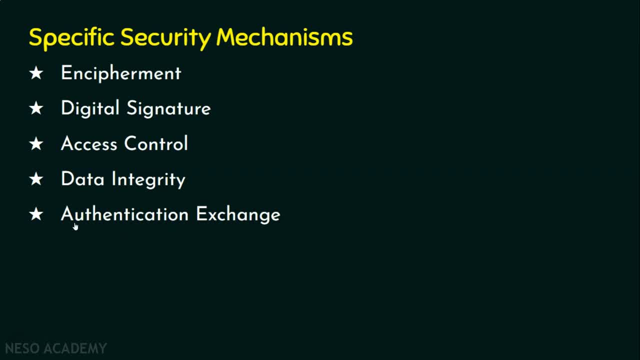 authentication purpose. We are done with the fifth security mechanism, the authentication exchange. Let's now move on to the next one, the traffic padding. Let's see the example in order to understand this traffic padding. In this example, let's assume Bob is going to send some data to Alice. 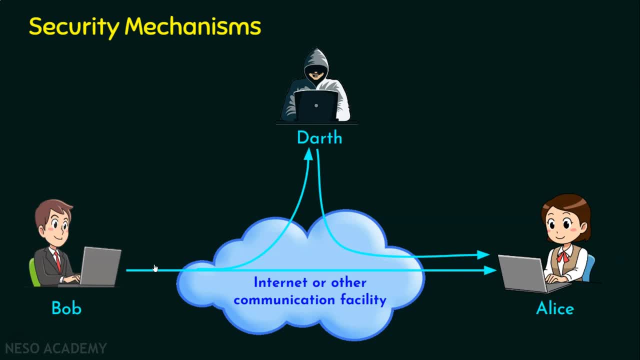 Now, let's say Bob and Alice have been connected and they have started communicating with each other. Now, for a certain period of time, Bob is not sending any data item, but still they are connected During when the data is not transmitted, Darth. 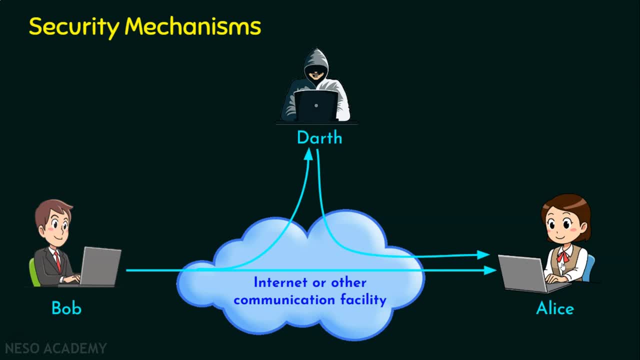 can come into action and he can send a false data stream to Alice, pretending that it is from Bob, In order to avoid this. what can be done When Bob and Alice are not sending any data item for a certain period of time in order to avoid the insertion of bits into the gaps in a data stream? we 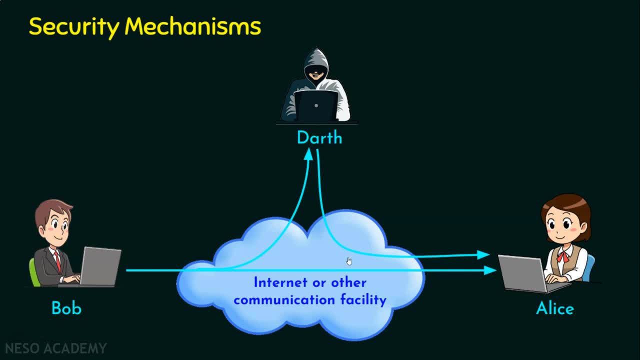 need to ensure that there is a dummy data stream that flows through the network in order to confuse them, But this dummy data stream may not have any impact with the receiver. Alice, This dummy data stream may be introduced into the network in order to confuse Darth, the attacker, not the receiver. 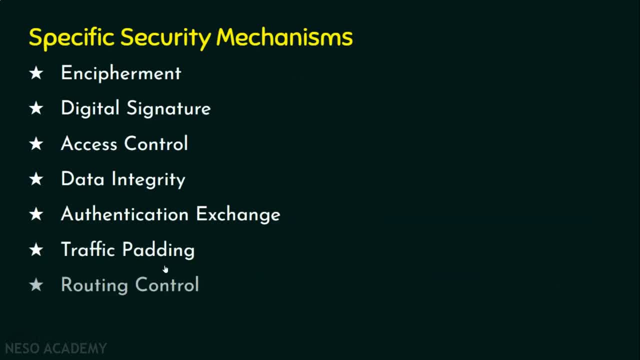 This is exactly traffic padding. Let's see the next security mechanism, which is routing control. We know the name itself says that we are going to control the routing process, and we know very well that routing is done by routers, and routers are not in our control. 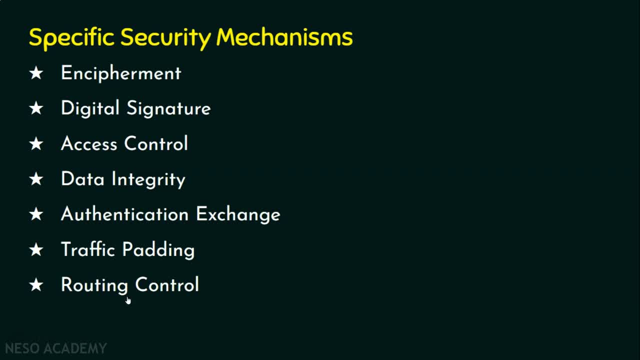 How to do then. routing control, Say, the data communication takes place in a certain route and if we suspect that the route is prone or vulnerable to attack, so what can be done? So we can physically secure the routes, especially when a breach of security is suspected, by informing that what? 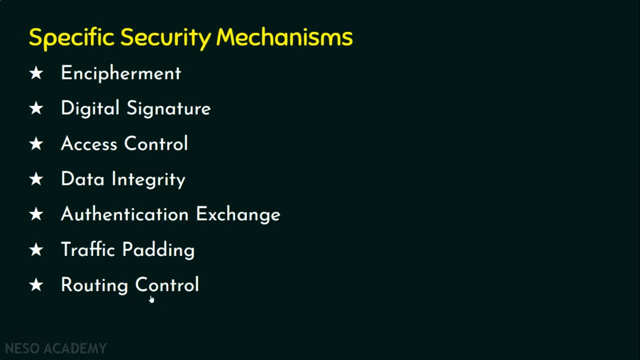 route the data must take in order to reach the destination. This is actually routing control In simple terms. when sender sends the data items on the network, it also specifies the route it should take in order to reach the destination, so that this data packet will not go in. 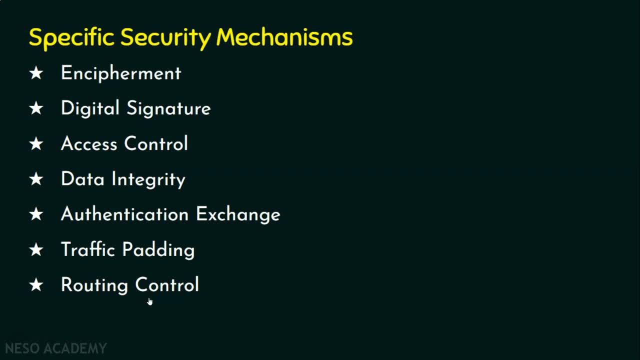 the hands of the attackers. So this is physically securing the routes. So routing control is one of the security mechanisms. Coming to the last security mechanism, which is notarization. What is notarization? Let's see the example. 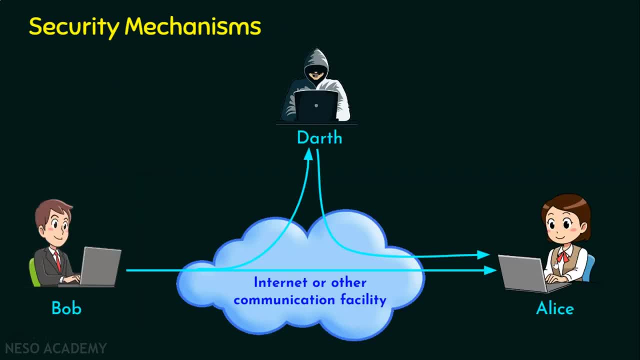 Say in this example, let's assume Bob and Alice are communicating and if there is a third party and we trust this third party, in other words, if that is a trusted third party? Please note, I am not talking about Darth, who is an attacker here. I am talking. 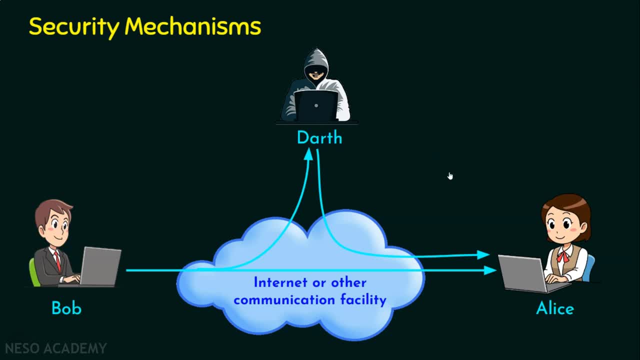 about a trusted third party which comes into action in order to resolve the disputes between Alice and Bob or in order to give some certificates to Bob, such a way that this certificate will help to reach Alice. So this is we call as notarization. 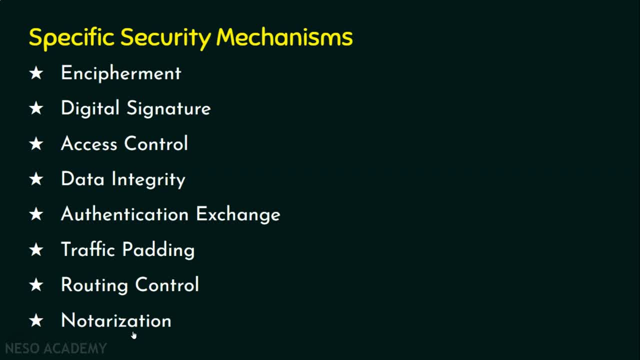 So, in simple terms, notarization means we are going to deploy some trusted third party. In reality say, if we want to access some secure servers, we have SSL certificates. right This? SSL certificates are issued by certificate authorities, where these certificate authorities are called as the trusted third parties. 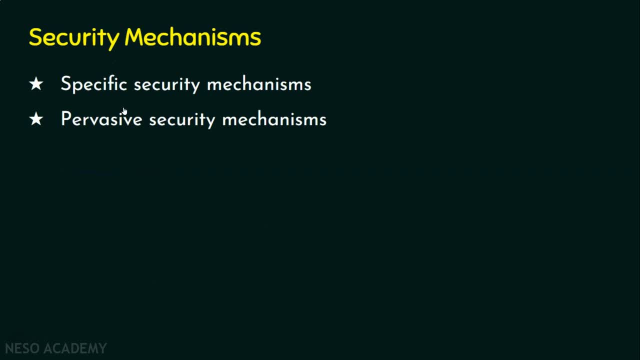 We are done with the first type, the specific security mechanisms. Let's now move on to the last type, the pervasive security mechanisms. We know specific security mechanisms incorporated into the appropriate protocol layers to provide some of the OSI security services. and coming to the pervasive security mechanism, this is not going to be incorporated to. 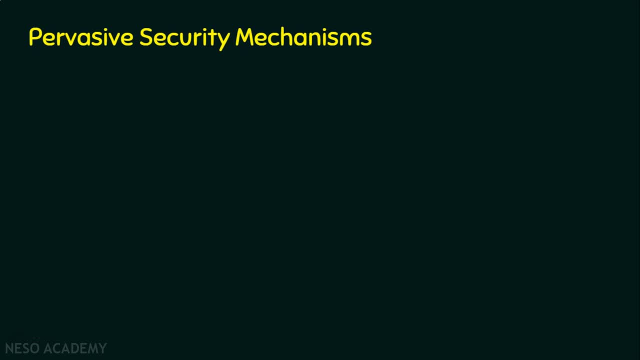 any particular layer or any particular service. This is a generalized security mechanism. Let's see the various security mechanisms under pervasive security mechanisms. The first one is trusted functionality. So this trusted functionality is perceived to be correct with some criteria. For example, we are going to enforce some security policies, and whenever. 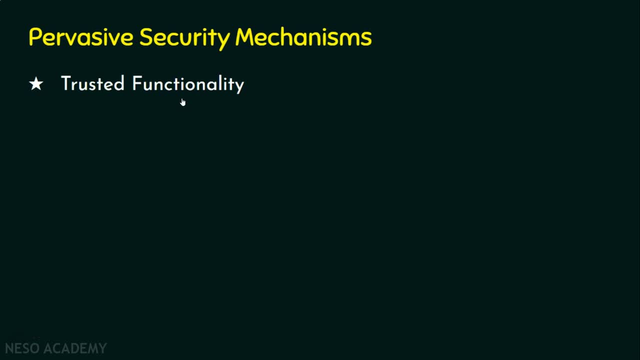 any action is carried out in the system or in the system resources, these security policies will help us to decide whether that action is a perfect one or not permitted one. So trusted functionalities, in simple terms, is perceived to be correct with respect to some criteria, for example security policies. 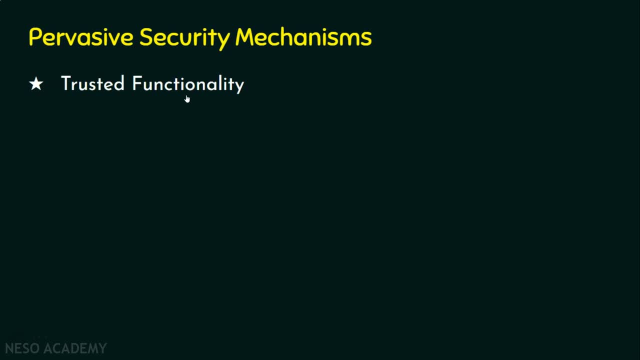 We are done with the first pervasive security mechanism. Let's now move on to the second one, which is security label. The name itself says that we are going to have some labels in order to achieve security, In order to access the resources, the security attributes. 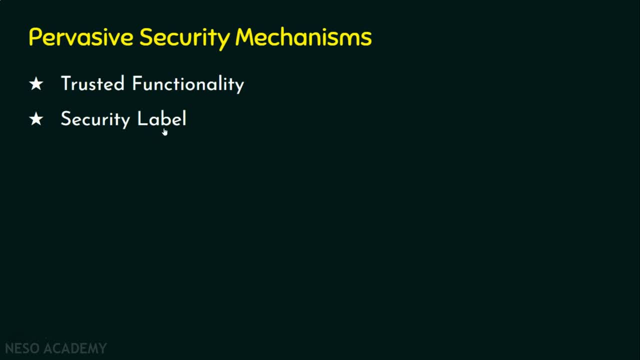 to resources. So security label helps us to identify we are doing the right thing. Coming to the third one, which is event detection. Event detection means whenever any activity is carried out in the secure system, events are generated. So these events can be a normal event or a non-normal event. 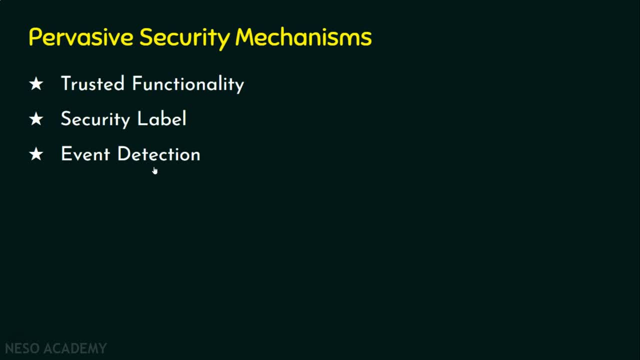 Or a suspicious event. So whenever any suspicious events are generated, we need to focus that. So in a secure system, we are going to focus on events where these events are security related events, which helps us to say whether a legitimate user. 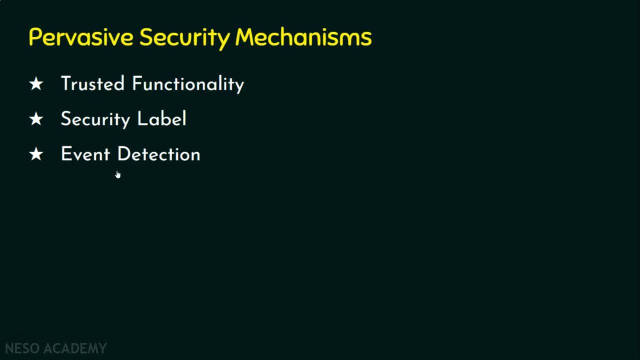 is accessing or creating the event, or it is done by the attackers or something is suspicious in the network. We are done with the third one, the event detection. Let's now move on to the fourth one, which is the security audit trial. We know whenever any activity is carried out in a secure system. 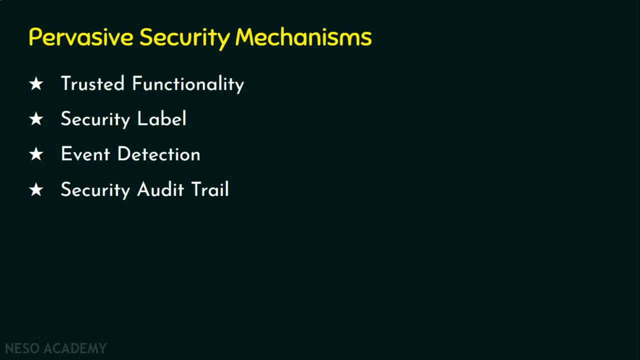 we need to collect certain data. All these data that are collected are used for doing security audits, So we are going to do some security audits based on the data that is collected. So what do you mean by this audit? We are going to do auditing.